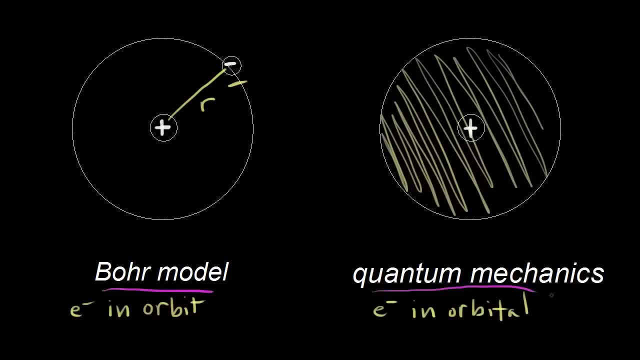 But quantum mechanics says we don't know exactly where that electron is And the Bohr model turns out to be incorrect And quantum mechanics has proven to be the best way to explain electrons in orbitals And we can describe those electrons in orbitals. 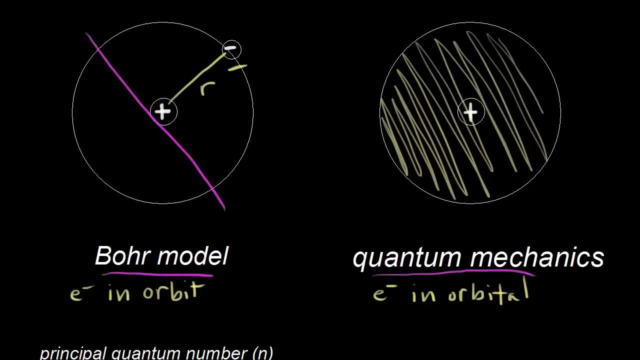 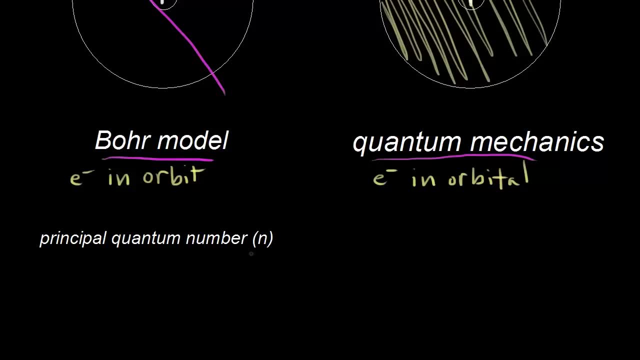 using the four quantum numbers, And so let's look at the first quantum number here. So this is called the principal quantum number, And the principal quantum number is symbolized by n. So n is a positive number, It's a positive integer. 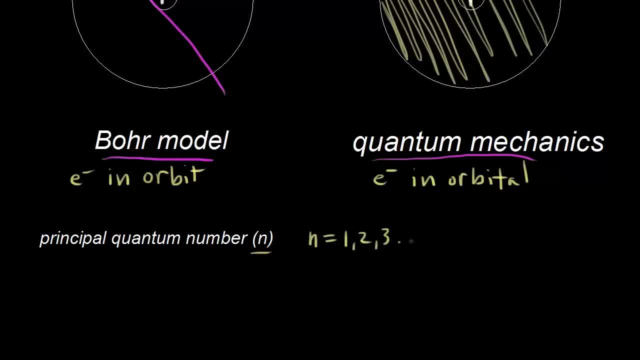 So n could be equal to one, two, three and so on. It indicates the main energy level occupied by the electron. So this tells us the main energy level, And you might hear this referred to as a shell sometimes, So we could say what kind of shell the electron is in. 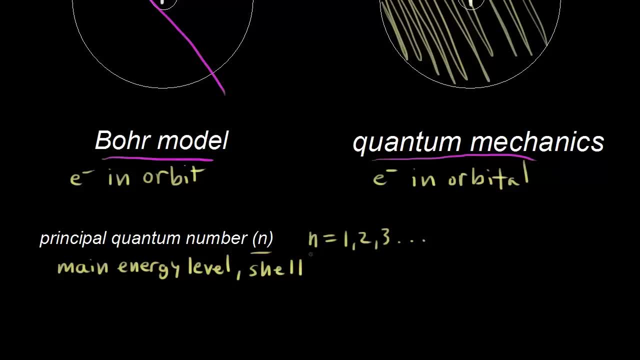 As n increases, the average distance of the electron from the nucleus increases. Therefore so does the energy. So for example- this was our nucleus right here, And let's talk about n- is equal to one. So for n is equal to one. 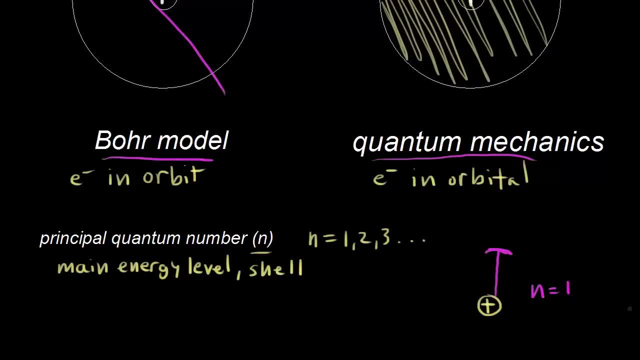 let's say the average distance from the nucleus is right about here. Let's compare that with: n is equal to two. n is equal to two means a higher energy level. So on average the electron is further away from the nucleus and has a higher energy associated with it. 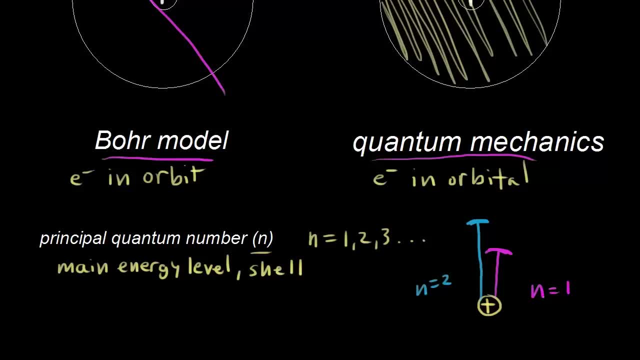 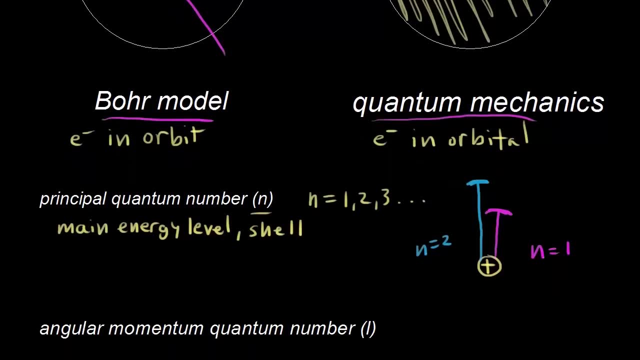 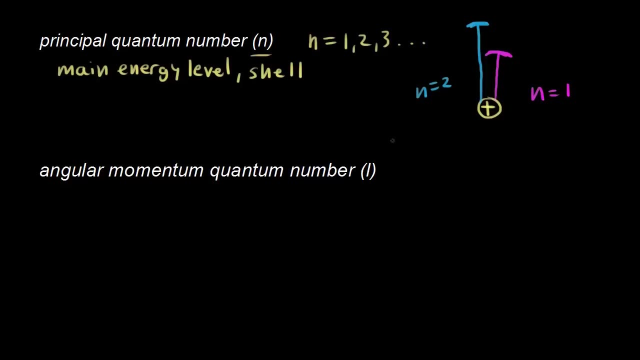 So that's the idea of the principal quantum number. You're thinking about energy levels, or shells, and you're also thinking about average distance from the nucleus, All right, our second quantum number is called the angular momentum quantum number. So the angular momentum quantum number. 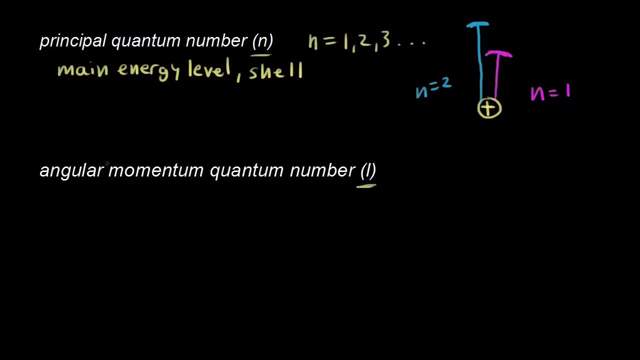 is symbolized by l, And l indicates the shape of the orbital. So this will tell us the shape of the orbital. Values for l are dependent on n, So the values for l go from zero all the way up to n minus one. 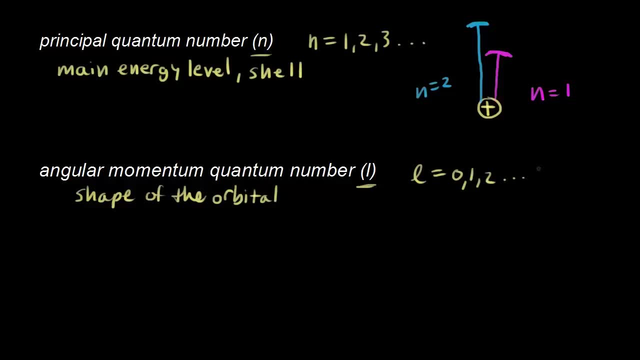 So it could be zero, one, two or however numbers, however values. there are up to n minus one. For example, let's talk about the first main energy level or the first shell. So n is equal to one. There's only one possible value you could get. 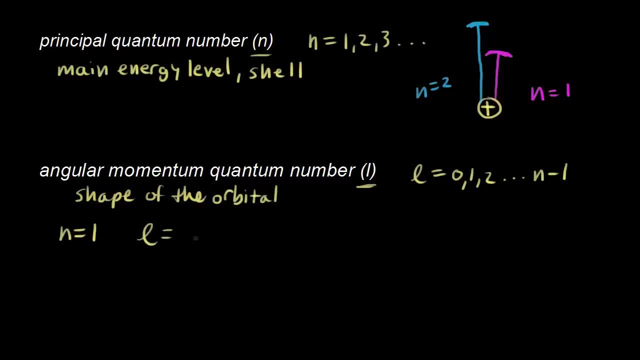 for the angular momentum quantum number, l. n minus one One is equal to zero, is equal to zero. So that's the only possible value, the only allowed value of l. When l is equal to zero, we call this an s orbital. 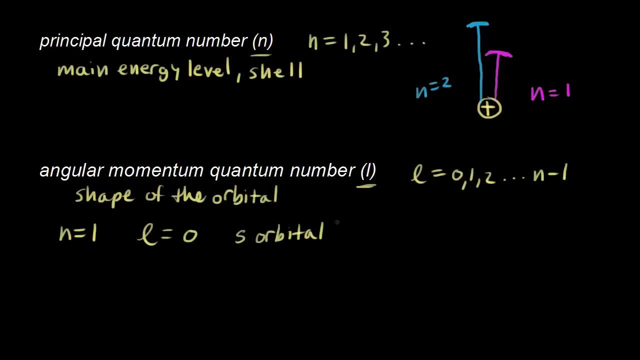 So this is referring to an s orbital, And the shape of an s orbital is a sphere. So we've already talked about that with the hydrogen atom. So just imagine this as being a sphere, right? So a three-dimensional volume here, So the angular momentum, quantum number l. 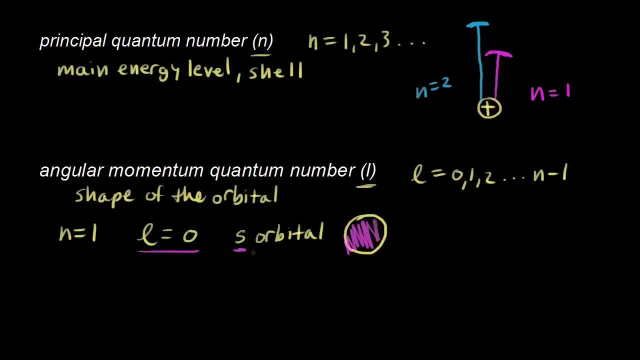 since l is equal to zero, that corresponds to an s orbital, So we know that we're talking about an s orbital here, which is shaped like a sphere, So the electron is most likely to be found somewhere in that sphere. Let's do the next shell. 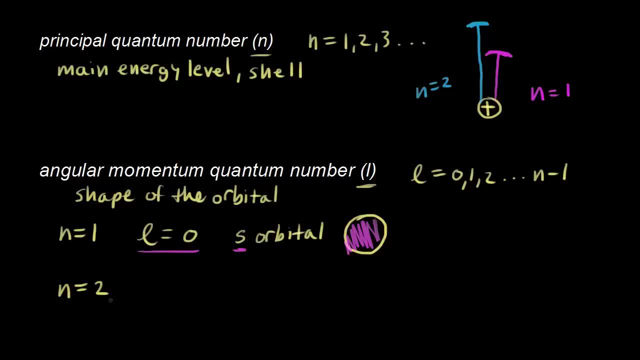 So n is equal to two. So if n is equal to two, what are the allowed values for l? So l goes zero, one, and so on all the way up to n minus one. So l is equal to zero, and then n minus one would be equal to one. 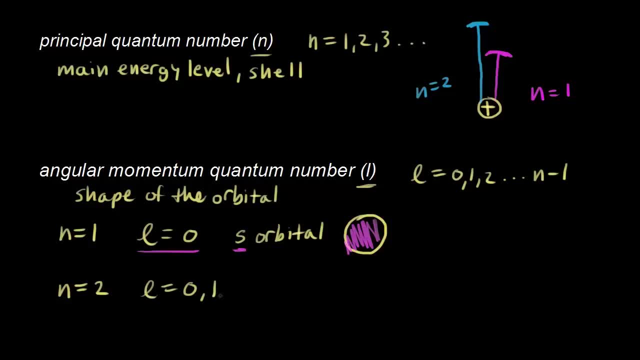 So we have two possible values for l. l could be equal to zero and l could be equal to one. Notice that the number of allowed values for l is equal to n. So, for example, if n is equal to one, we have one allowed value. 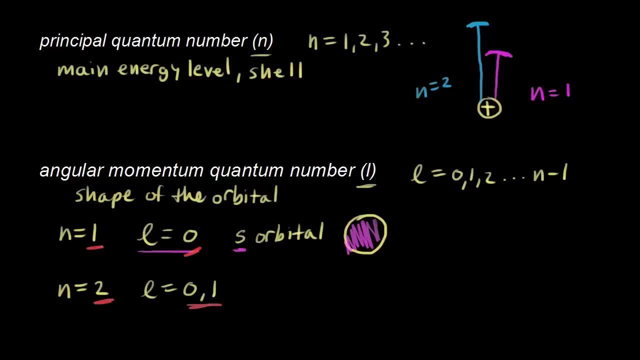 If n is equal to two, we have two allowed values. All right, we've already talked about what l is equal to zero, what that means. So l is equal to zero means an s orbital shaped like a sphere. But now in the second main interval, 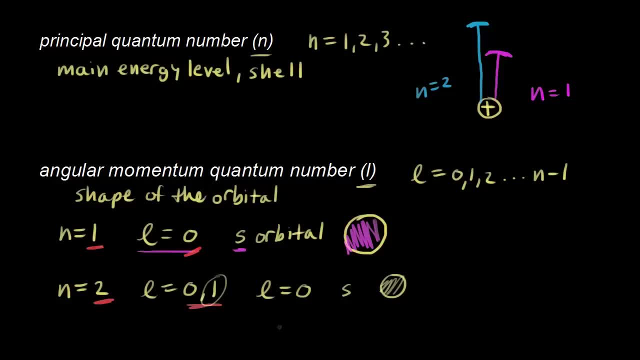 the energy level or the second shell. we have another value for l, So l is equal to one. And when l is equal to one we're talking about a p orbital. So l is equal to one means a p orbital, And the shape of a p orbital is a little bit strange. 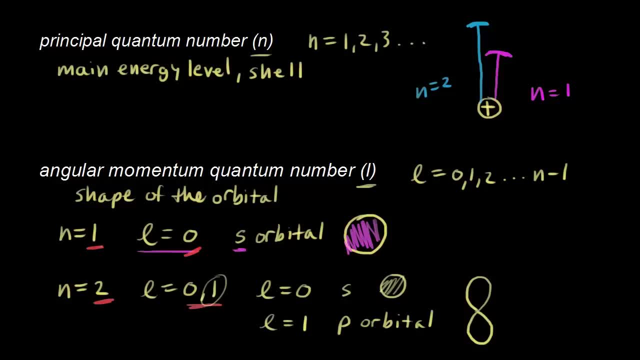 So I'll attempt to sketch it in here So you might hear several different terms for this. So imagine this is a volume, right? So this is a three-dimensional region in here, So you could call these dumbbell-shaped or bow-tie, whatever makes the most sense to you. 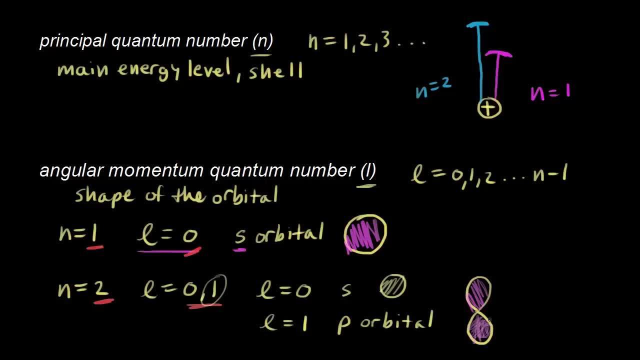 But this is the orbital. This is the region of space where the electron is most likely to be found, if it's found in a p orbital. here Sometimes you'll hear these called sub-shells, right, So if n is equal to two, if we call this a shell, 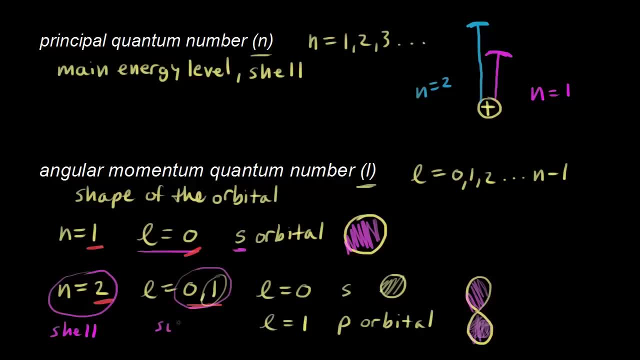 right, if we call this a shell, then we would call these sub-shells. All right, so these are sub-shells. here And again we're talking about orbitals. L is equal to zero is an s orbital. L is equal to one is a p orbital. 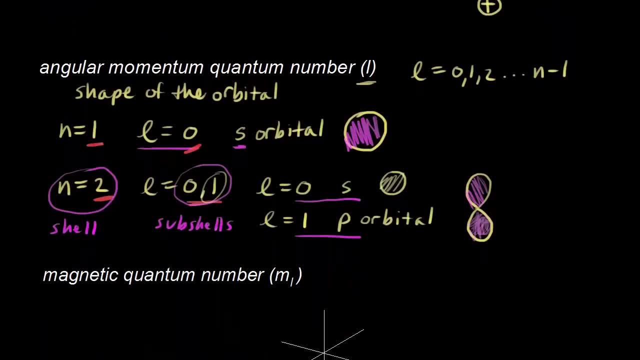 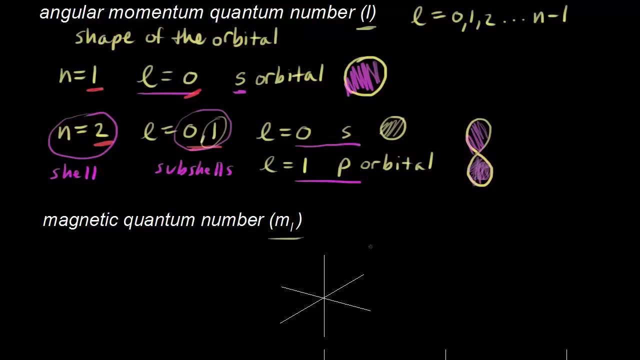 Let's look at the next quantum number. So let's get some more space down here. So this is the magnetic quantum number symbolized by m sub l here. So m sub l indicates the orientation of an orbital around the nucleus. So this tells us the orientation of that orbital. 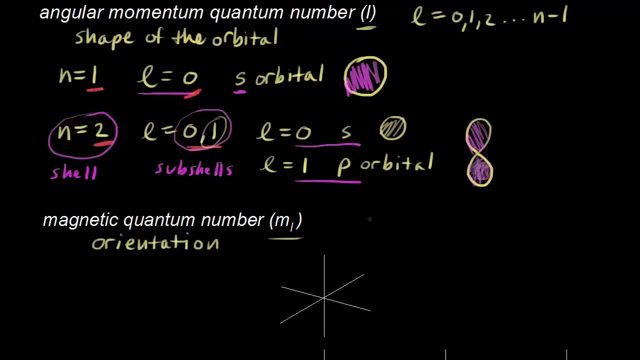 And the values for m l depend on l. So m? l is equal to any integral value that goes from negative l to positive l. All right, so that sounds a little bit confusing, Let's go ahead and do. the example of l is equal to zero. 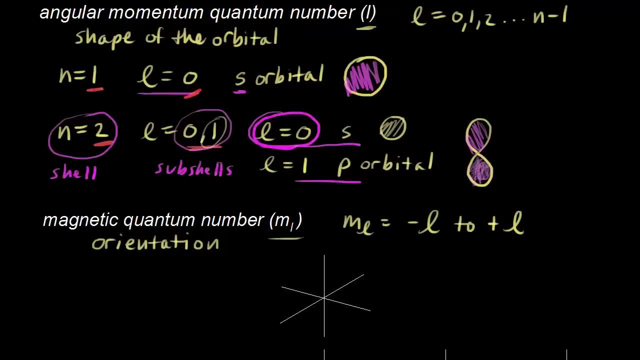 All right, so l is equal to zero up here. So let's go ahead and write that down here. If l is equal to zero, what are the allowed values for m? l? There's only one. all right, There's only one. 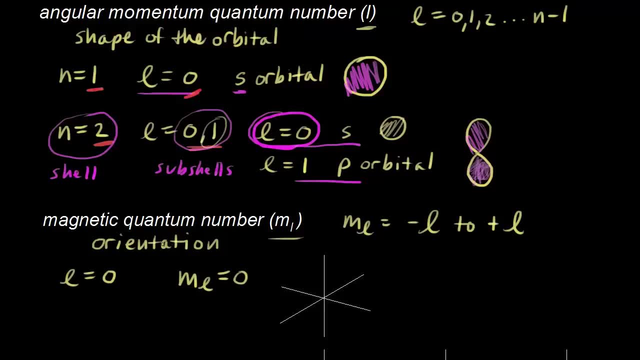 The only possible value we could have here is zero. So when l is equal to zero, when l is equal to zero, let me use a different color here. So if l is equal to zero, we know we're talking about an s orbital right. 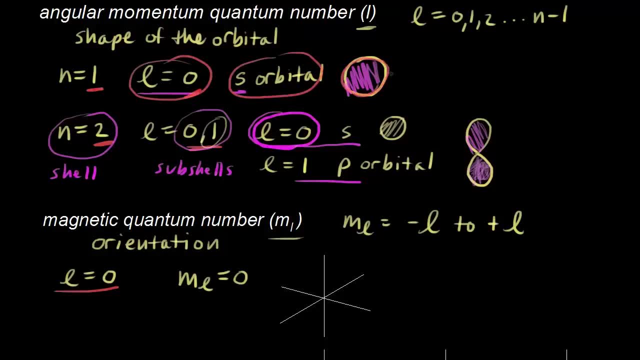 When l is equal to zero, we're talking about an s orbital which is shaped like a sphere And if you think about that, we have only one allowed value for the magnetic quantum number That tells us the orientation. So there's only one orientation for that orbital. 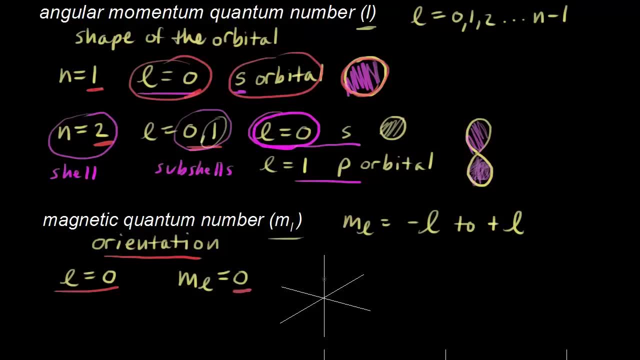 around the nucleus, And that makes sense because a sphere has only one possible orientation. So if you think about this as being an x, y, z axis, excuse me, and if this is a sphere, there's only one way to orient that sphere in space. 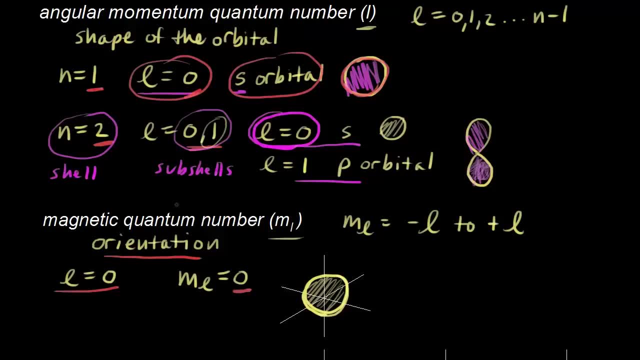 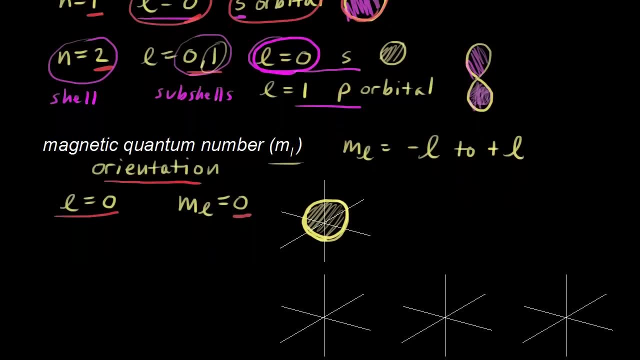 And so that's the idea of the magnetic quantum number. All right, let's do the same thing for l is equal to one, All right, so let's look at that now. So if we're considering l is equal to one, let me use a different color here. 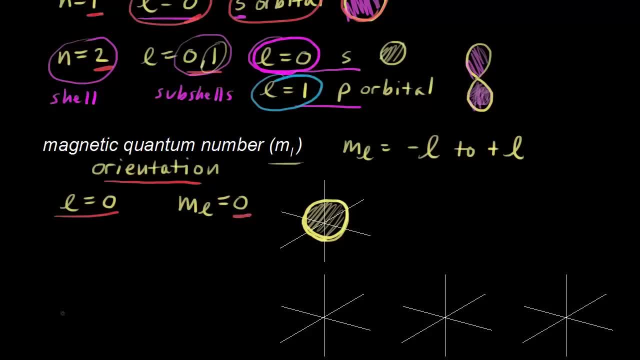 So l is equal to one. Let's write that down here. If l is equal to one, what are the allowed values for the magnetic quantum number? So ml is equal to. this goes from negative l to positive l, So any integral value from negative l to positive l. 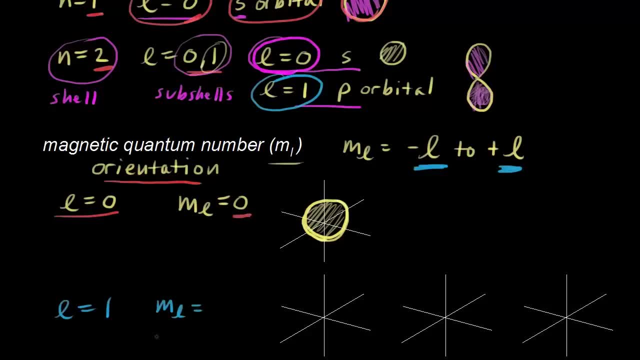 Well, negative l would be negative one. So let's go ahead and write this in here, So we could have negative one, zero and positive one. So we have three possible values. So when l is equal to one, we have three possible values. 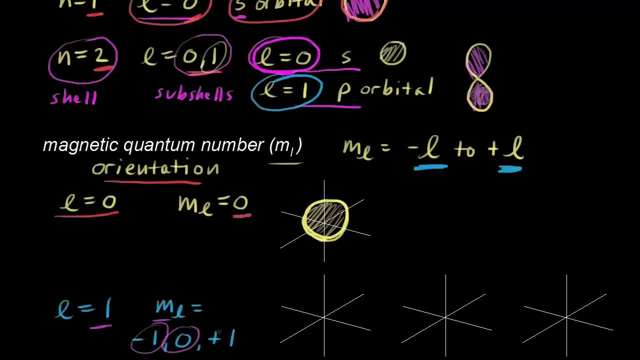 for the magnetic quantum number, So one, two and three. The magnetic quantum number tells us the orientations, So the possible orientations of the orbital or orbitals around the nucleus here. So we have three values for the magnetic quantum number. That means we get three different orientations. 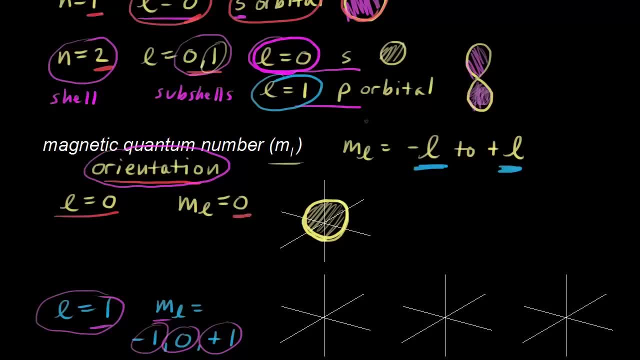 And we already said that when l is equal to one One, we're talking about a p-orbital, and a p-orbital is shaped like a dumbbell here. So we have three possible orientations for a dumbbell shape. So if we went ahead and put some 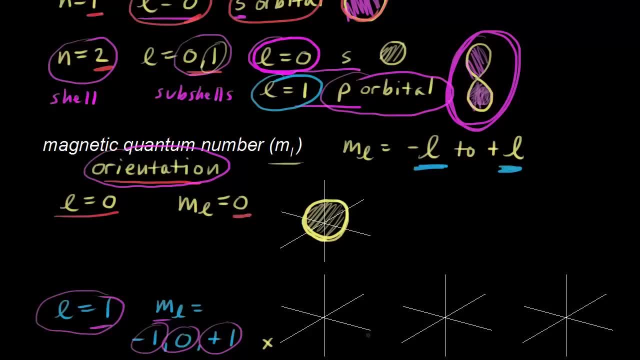 marked these axes here. let's just say: this is x-axis, y-axis and the z-axis here. So we could put a dumbbell. we could put a dumbbell on the x-axis like that. So again, imagine this as being a volume. 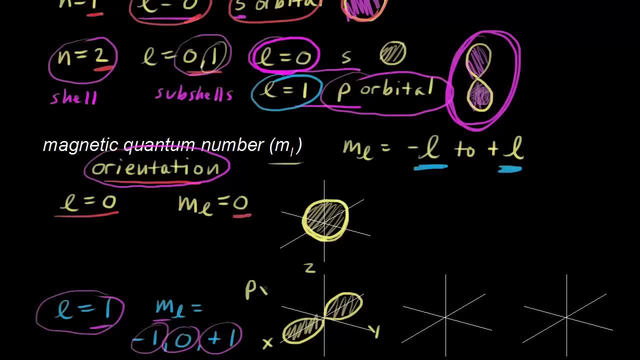 This would be a p-orb. we'd call this a p-x-orbital. It's a p-orbital and it's on the x-axis. here We have two more orientations, So we could put again: if this is x. 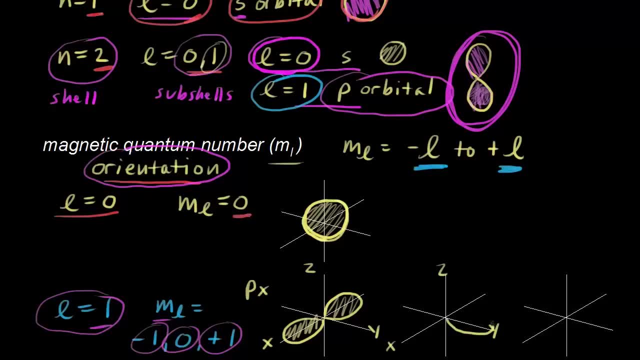 this is y and this is z. we could put a dumbbell. we could put a dumbbell here on the y-axis. So there's our second possible orientation. And then, finally, if this is x, this is y and this is z. 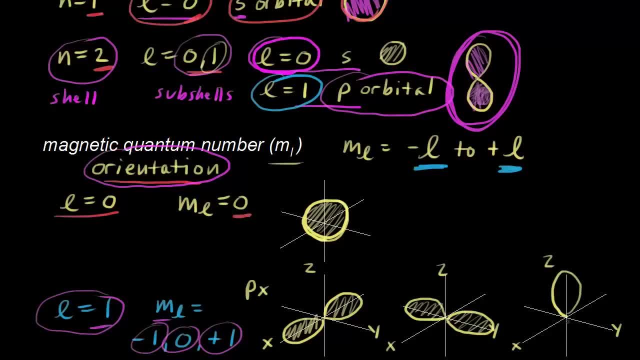 of course we could put a dumbbell on the z-axis like that. So this would be a p-z-orbital. So we could write a p-z-orbital here and then this one right here would be a p-y-orbital. 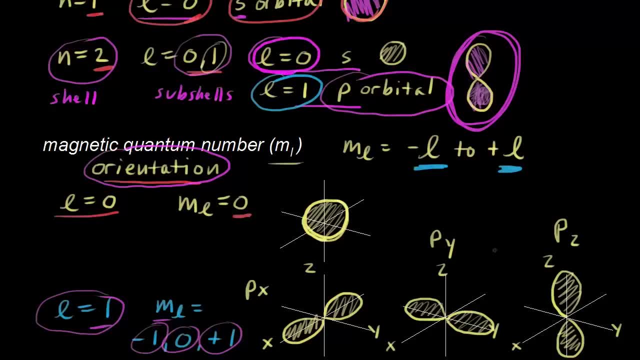 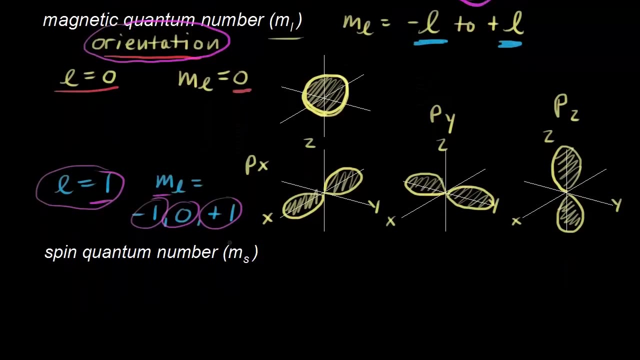 So we have three orbitals, we have three p-orbitals here, All right, so one for each axis. All right, let's go to the last quantum number. So the last quantum number is the spin quantum number. So the spin quantum number is m sub s here. 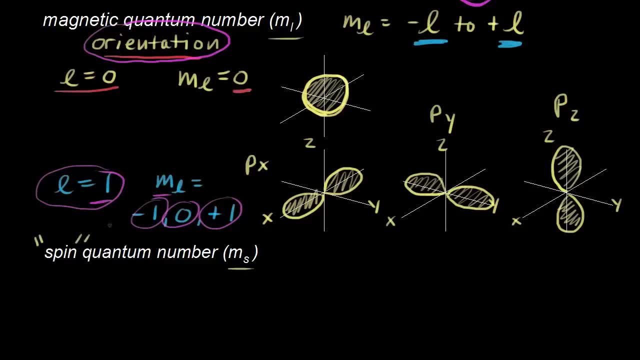 And so what it says here, when it says spin- I'm gonna put this in quotations- like this- seems to imply that an electron is spinning on an axis. So that's not really what's happening, but let me just go ahead and draw that in here. 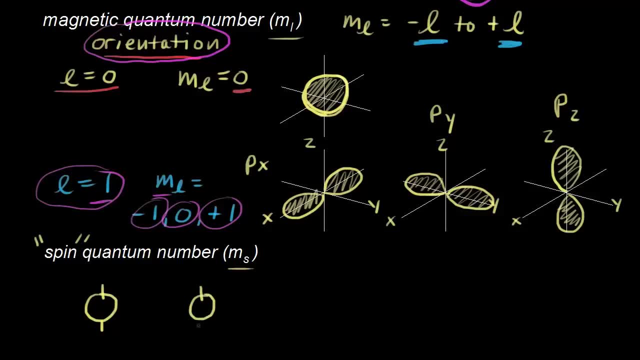 So I could have an electron- let me draw two different versions here. So I could have an electron spin like a top, if you will, this way, or I could have an electron spin around that axis going this way And again, this is not actually what's happening. 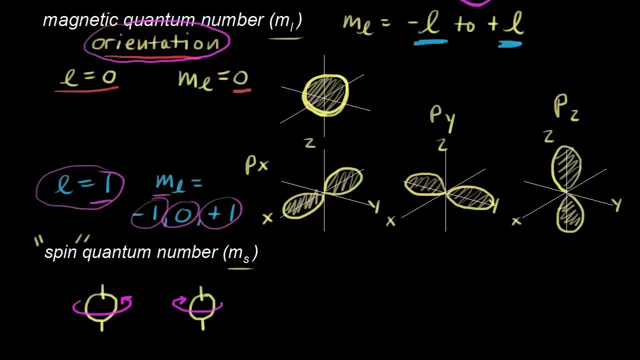 in reality The electrons don't really spin on an axis like a top. but it does help me to think about the fact that we have two possible values for the spin quantum number, So you could spin one way, So we could say the spin quantum number. 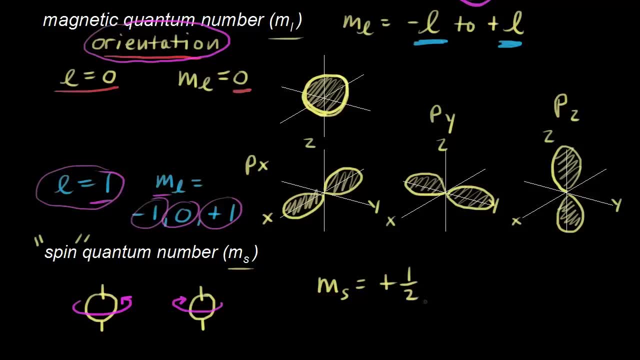 is equal to positive 1 1⁄2. So usually you hear that called spin up, So spin up, and we'll symbolize this with an arrow going up in later videos here. And then the other possible value for the spin, quantum number. 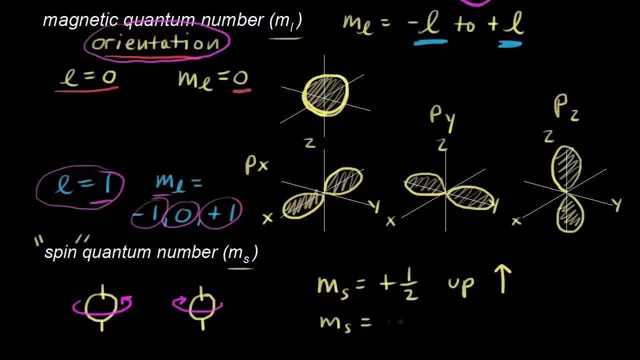 so the spin quantum number is equal to negative 1 1⁄2.. So you usually hear that referred to as spin down and you could put an arrow going down. So again, electrons aren't really spinning in a physical sense like this.